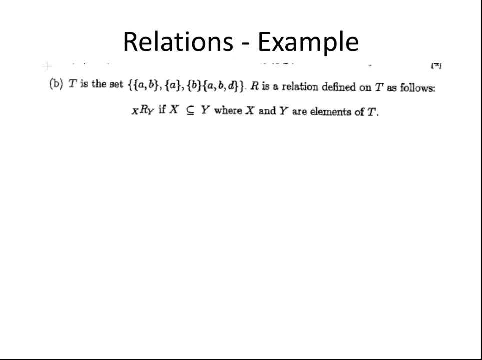 So let's draw the relation first. So start off here, up at the top, I'm going to draw this one here And I'm going to draw another node there, another node there and another node there. So up at the top, I'm going to have. 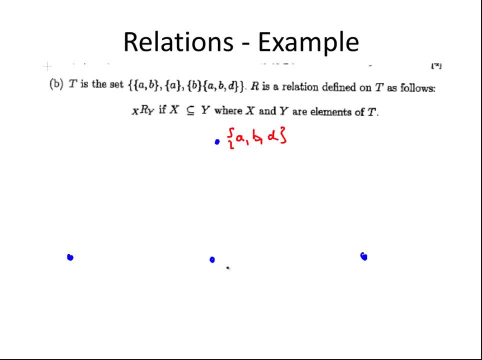 A, B and D. Down here I'll have A and B, Here I'll have B, And over here I'll have A. Okay Now. so let's put in the directed edges. So A is a subset of A, B, D. 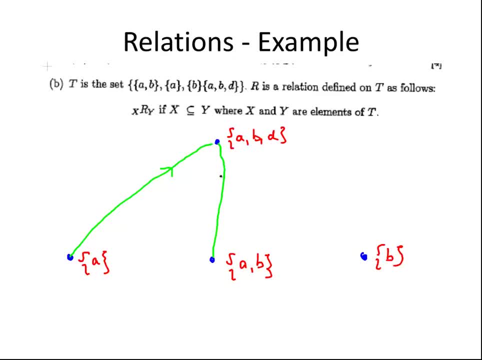 A and B is a subset of A, B, D, And B Is a subset of A, B, D. So those are a couple of our relations. A is also a subset of A and B, As is B. That's a subset of A and B. 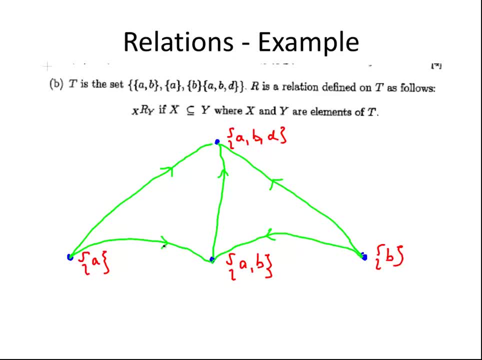 So two more directed edges there. Now to finish off, just remember that everything is a In set theory, that everything is a subset of itself. So we have one more directed edge pointing back at each vertex. So So A is a subset of A. 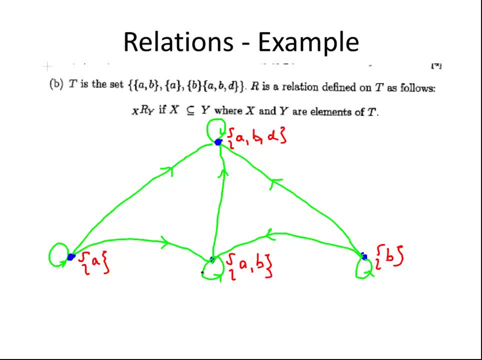 A, B is a subset of A, B, A, B, D is a subset of A, B, D, And B is a subset of B. Okay, So that's our directed graph, our digraph. Now what we have to do is decide if it is reflexive. 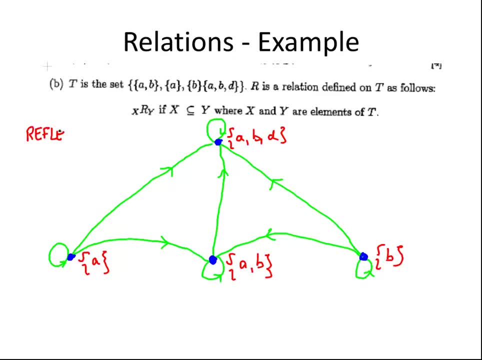 Well, I'm actually already after answering that one already. Uh, The reason is that every First off, every node here has an edge directed back at itself. Okay, And again, as I just said there previously, everything is a subset of itself in set theory. 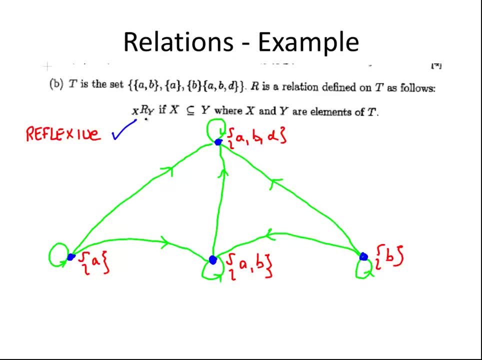 So in this case it is reflexive. Okay, Now is it symmetric? So if X is a subset of Y, is Y necessarily a subset of X? In that case it would be symmetric. Well, A is a subset of X. 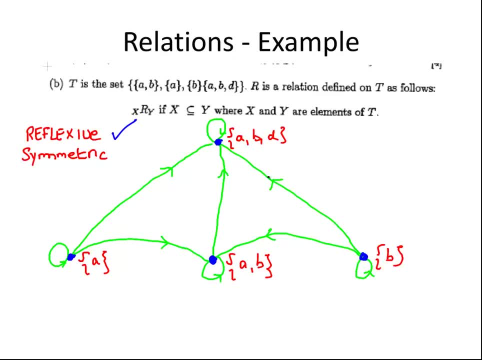 A is a subset of A and B. Well, A and B is not a subset of A. Likewise, in every other sort of pairing, the relationship only works one way. So in this case we do not have a symmetric relationship. 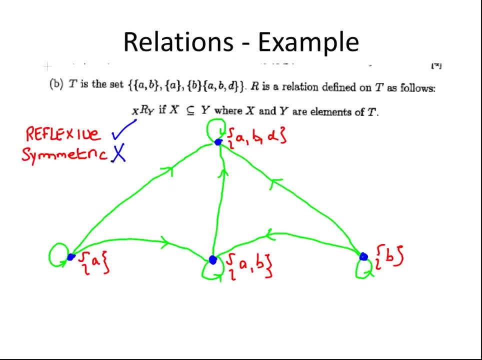 If one is a subset of the other, it doesn't necessarily work in reverse, Not necessarily work in reverse. So is it transitive? Is it transitive So if A? Now Let's just sort of disregard the fact that A is a subset of A, B, D, directly. 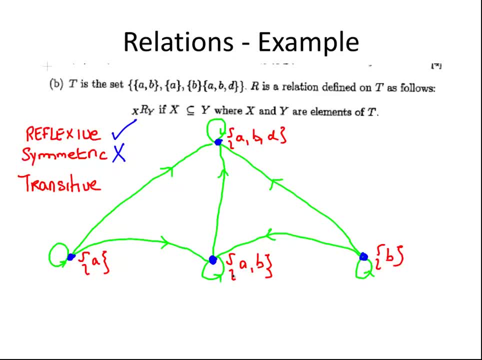 So let's just disregard this edge for a minute. A is a subset of A and B, And A and B is a subset of A B D. Does that make A a subset of A B D? Yes, it does. 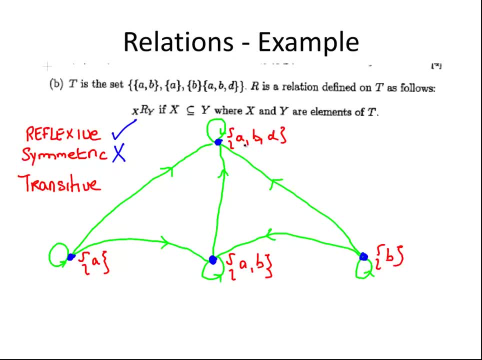 Likewise for every other sort of way you can look at it. B is a subset of A and B, And A and B is a subset of A, B, D. So this relationship is transitive. Okay, So it's symmetric. 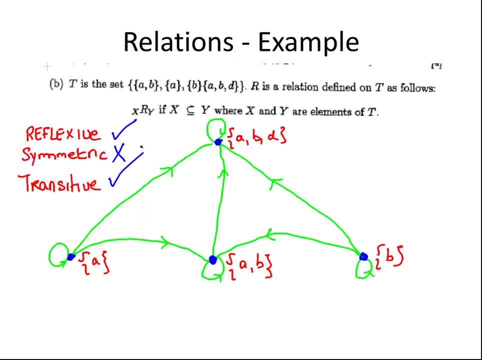 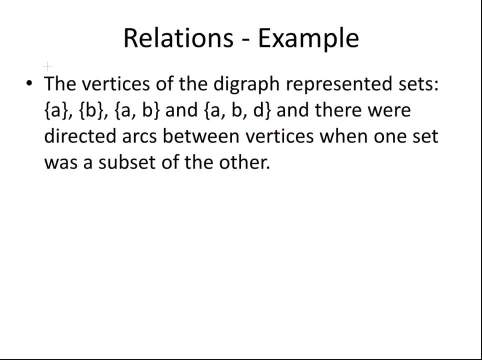 It's not symmetric, But it is reflexive. It's reflexive and transitive. Now we are asked to find out one more thing. Is it a partial order? So I'm just going to go to the next page here for a second. 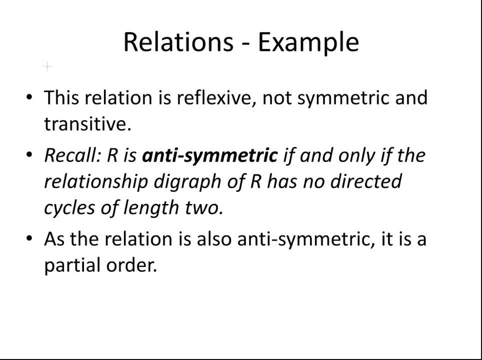 Okay, That's good. So the relationship is reflexive, not symmetric, and transitive. Now recall a relationship: R is anti-symmetric if, and only if, the relationship diagraph of R has no directed cycles of length 2. That's a sort of quick way we can. 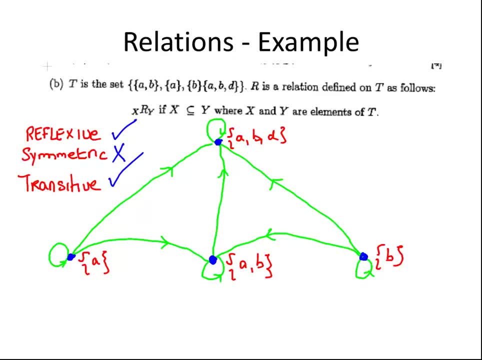 Just check. So in this case there are no directed cycles of length 2.. So a directed cycle has to be, Has to begin and end at the same node. I'll just sort of Let's put in just sort of counter example of what a directed cycle of length 2 would look like. 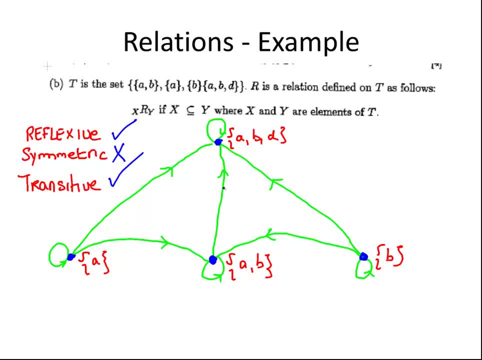 Just disregard, That's not a. So we have a This one here, This one here, This directed edge here And another edge that will go back. That would be a directed cycle of length 2. So there are actually none of those in the 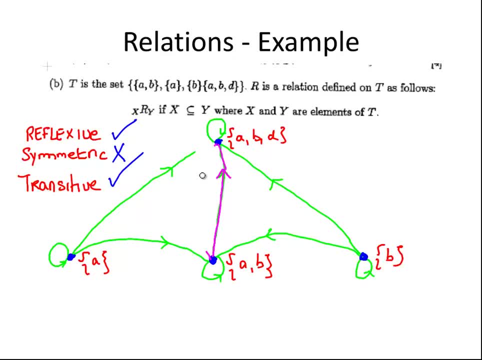 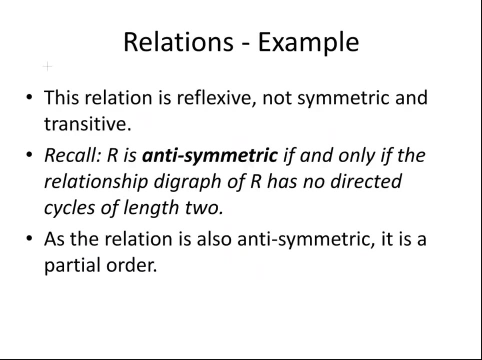 There are actually none of those in the diagraph, So we don't have any. So we can say that the Oops, We can say that the relationship is symmetric. Okay, So I've just directed the diagraph there, But anyway,